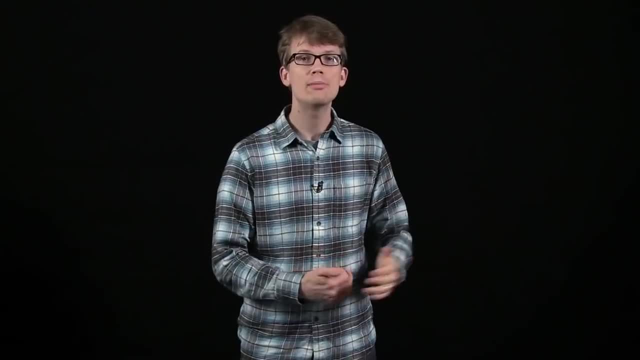 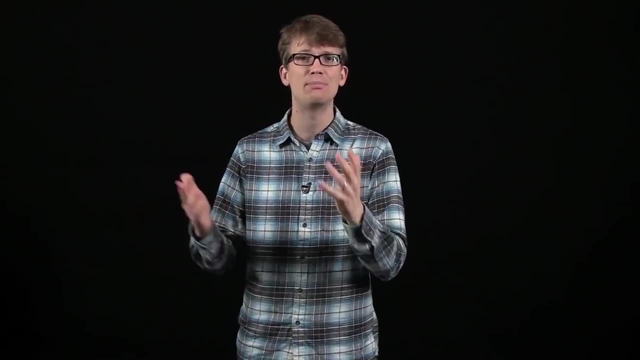 We often hear about all the different ways that our behavior is affecting the biosphere- extinctions, climate change, deforestation, acid rain, desertification, pollution and more. But you're asking: oh well, why are all those things bad? What's going on? 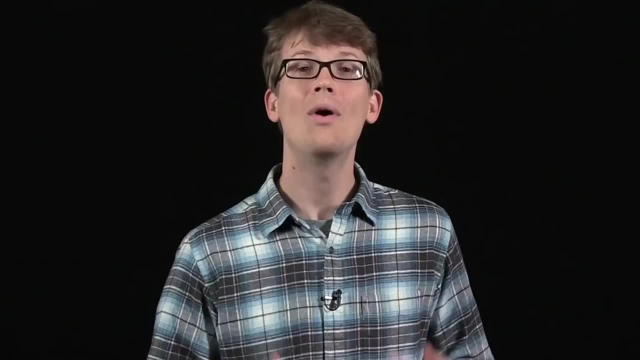 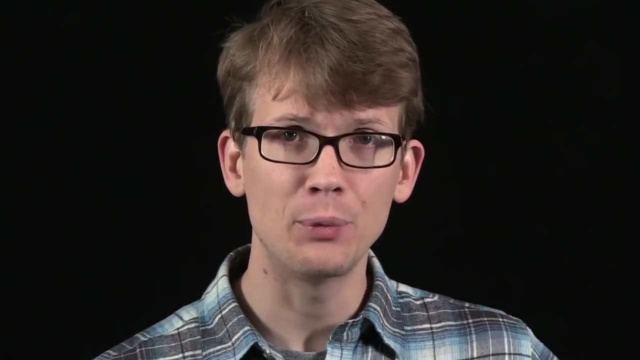 How is this stuff turning the Earth into sausage? I don't understand. Well, I do understand, which is why I'm qualified to make this video, So let me lay it on you. The services that ecosystems provide for us, all, the dirty work they do, can be broken up into four different categories. 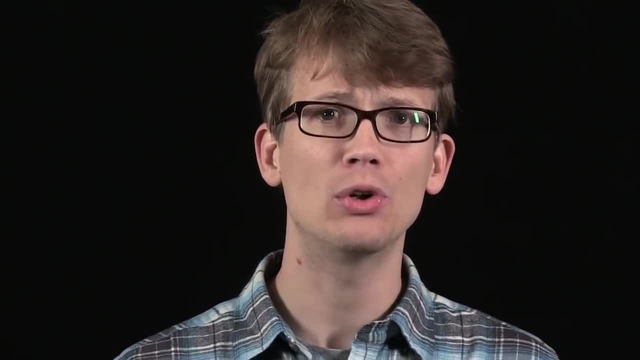 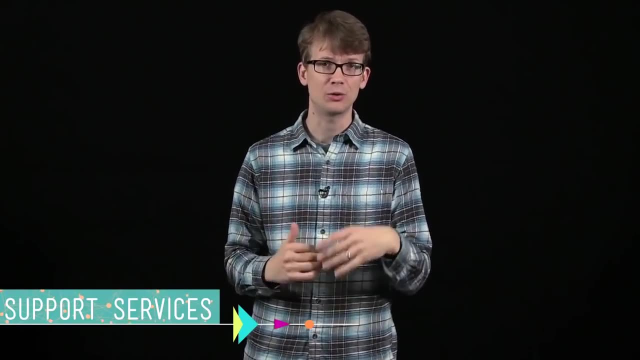 There are things that we could never eat. There are things that we could never, ever, ever duplicate or work around, no matter what kind of smarty-pants technology we come up with. First, healthy ecosystems provide support services that create and replenish the foundation of the Earth's biological systems. These services include recycling all of the compounds that are necessary for life through the carbon, water, nitrogen and phosphorus cycles. They also include other processes we've talked about before, like forming new soils and producing atmospheric oxygen. Some ecosystems contribute more to these services than others. 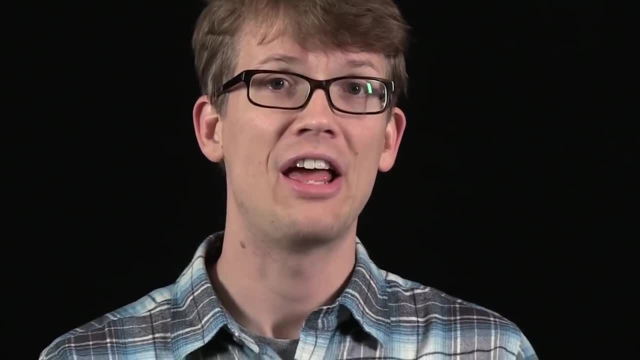 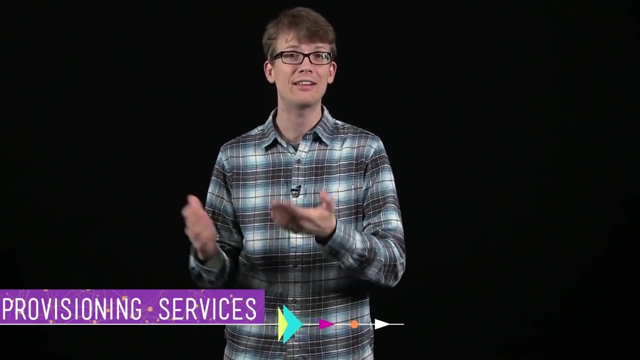 but none of them can get these basics done. Two ecosystems also perform provisioning services, giving us the raw materials we need to live like. the ocean provides food in the form of fish, sticks and stuff, And rivers and aquifers and other freshwater sources give us water. 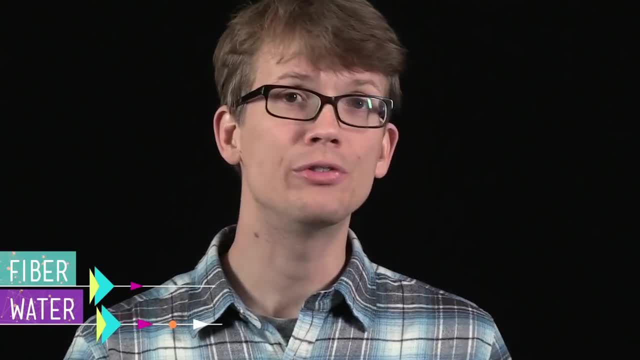 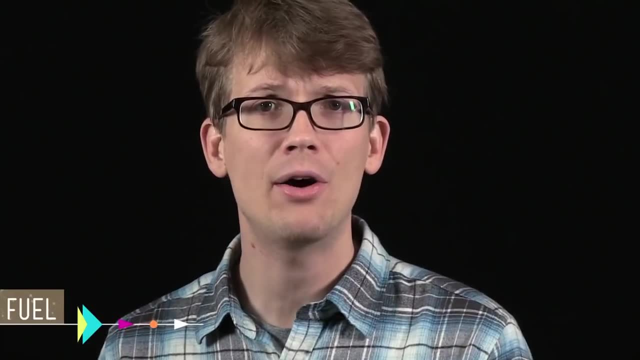 Plants and animals also yield all kinds of fiber that we use for clothing and shelter, and all around us we find sources of fuel, whether it's biomass in the form of grasses or wood, hydropower in the form of flowing water or the carbon locked in millions of years old trees and trees. But I'm getting ahead of myself. Ecosystems also perform super important regulating services, moderating many of the Earth's systems that can get dangerous if they get out of whack, Like as we learned in biology. fungi and other organisms take on the task of decomposing dead things and poop. 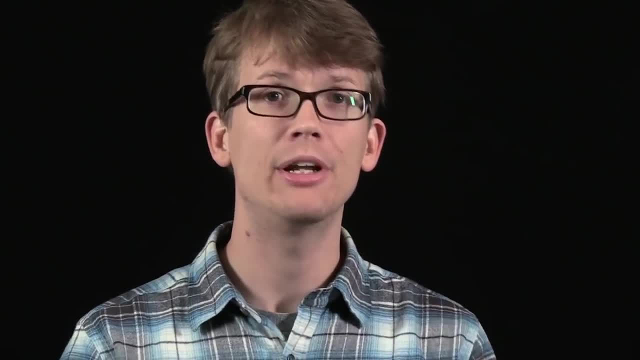 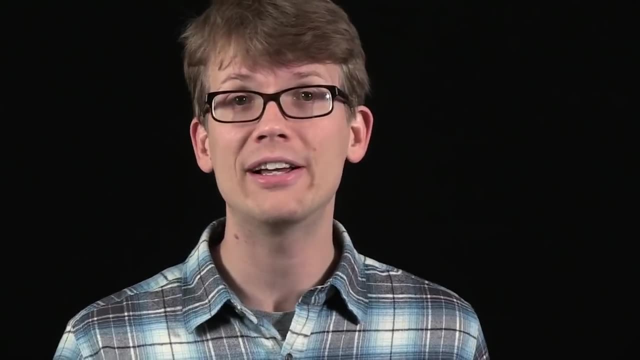 Meanwhile, plants help filter the water you drink and the air you breathe and provide flood control, and they also absorb all that carbon you exhale and that your car belches out, which in turn helps regulate the climate. And finally, number four: ecosystems are just kind of awesome. It's nice to be surrounded by happy plants and critters doing their business. Nice, robust ecosystems give us places to play, scenes to inspire us and things to just discover and learn about. These are- they're less tangible but still important cultural services. 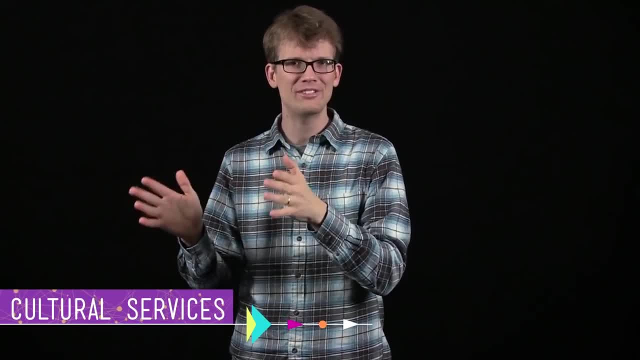 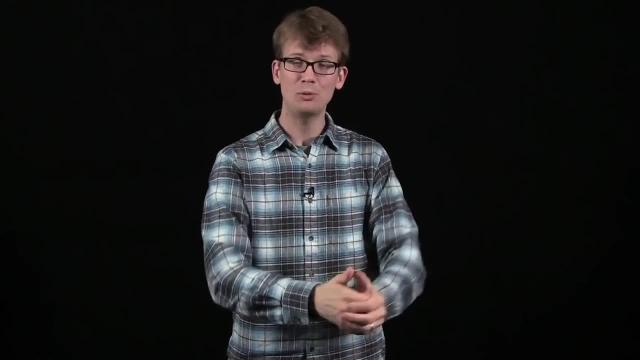 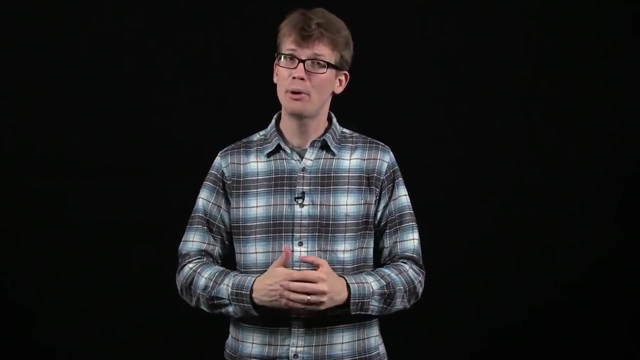 An interesting thing about ecosystem services is that economists actually can and do calculate the monetary value they provide for humanity. If, for example, we had to do all of the things that ecosystems do for us, it would cost us 46 trillion dollars per year. which is a lot considering that the output of the global economy is 66 trillion dollars per year. So, yeah, we should be happy that we're not. we don't have to pay for all that. But you'll notice that I keep saying that ecosystems can only serve up all this awesome sauce if they are intact. By that I mean they specifically have to have their biodiversity intact, because ecosystems are just a bunch of living and non-living things working together, so unless their living parts are healthy, they're basically just rocks and weather. The main reason biodiversity is so important is that it makes ecosystems more resilient to that never-ending change we talked about a few weeks ago. Ecosystems with high biodiversity are way more resilient to disturbances than those with low biodiversity. In a high biodiversity system, if you take one species out of the mix, it's less likely that the ecosystem will collapse. Take a hectare of Amazonian rainforest. In that little patch of land there are more different species of plants and animals than there are in all of Europe. So if a species of insect goes extinct, there's less risk that the whole house of cards will fall than, say, in the Sonoran Desert. 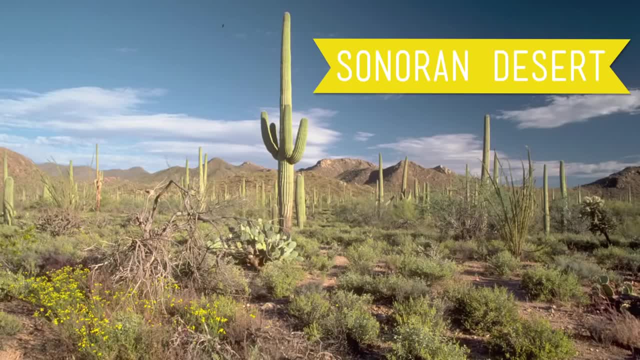 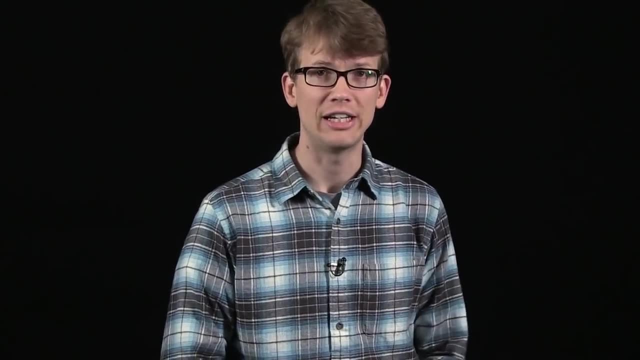 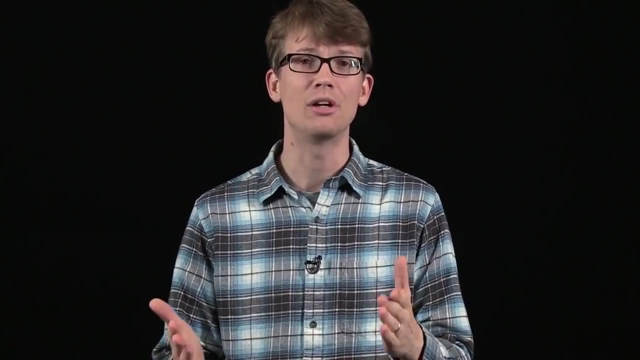 where there are very few organisms. so the disappearance of one species could affect the entire ecosystem. So the best way to understand our impacts on the environment is through how we affect biodiversity. Unfortunately, it turns out that we've been doing a really bang-up job of endangering some of the highest biodiversity ecosystems on the planet. 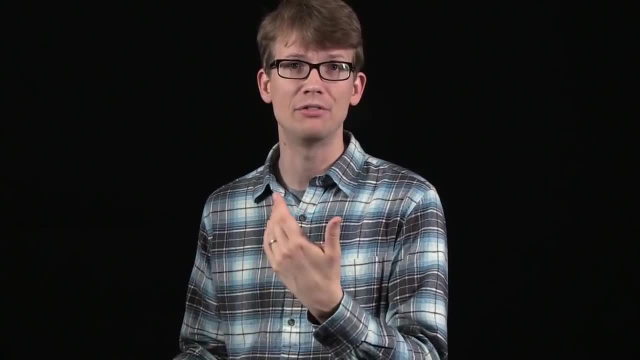 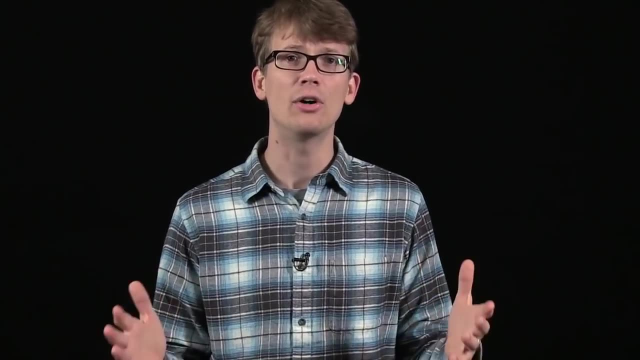 In some cases we're having impacts on the organisms themselves directly. In other cases we're affecting biodiversity Indirectly by creating one or two changes in that ecosystem that cascade into all kinds of problems for living things. First, let's look at that hectare of Amazonian rainforest again. 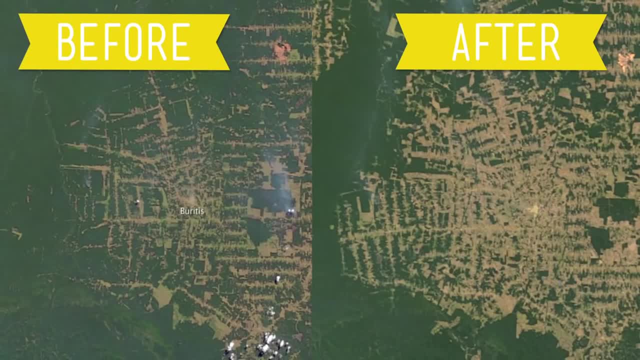 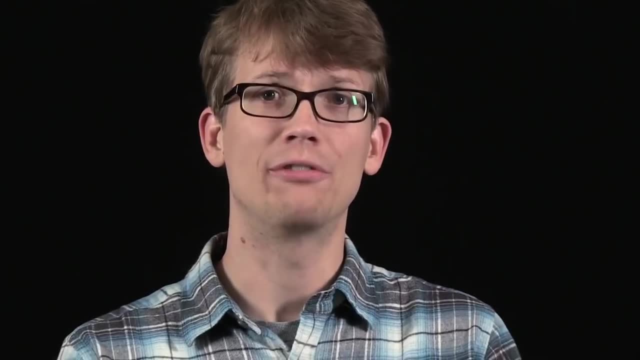 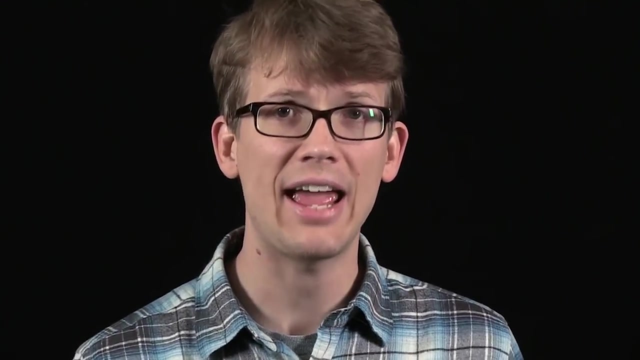 because, even though it's one of those super resilient ecosystems, we're having serious impacts on it. How Well? first, by removing a lot of what makes a forest a forest: Trees. According to some estimates, we're clear-cutting around 8,000 hectares of trees a day to provide land to graze cattle on. 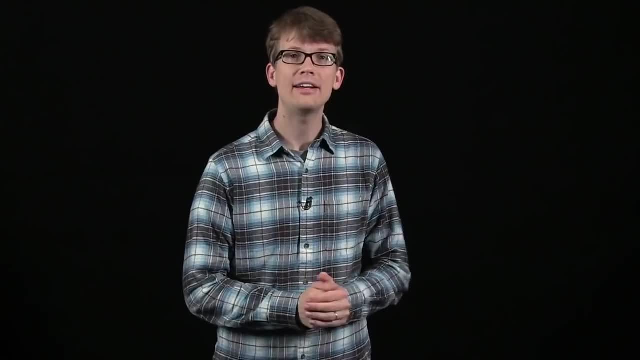 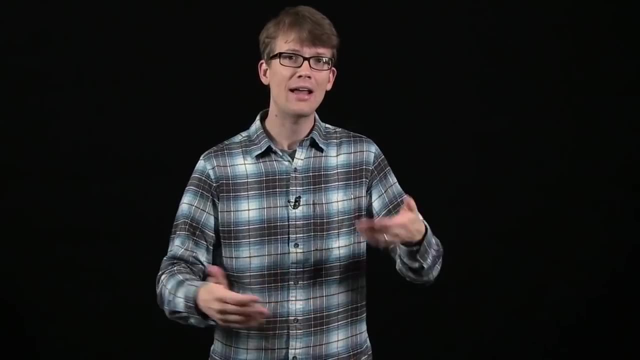 and to harvest wood to make coffee tables or whatever. When you cut down a hectare of rainforest, suddenly a place where a few thousand species used to live turns into a place where just a handful of species live: Some grass, some weeds, maybe some rats or mice, some insects and, you know, some cows. Because, man, we love cows. And when you take out so many of the living things on that hectare of land, a bunch of things happen. For starters, you're not just affecting that ecosystem, but neighboring ecosystems as well. For instance, all those trees that were cut down provided the service of regulating the flow of all that rain. that rainforests get, not only by absorbing some of it, but also by slowing down runoff, letting the water seep into the soil before slowly making its way into streams and rivers and ultimately the ocean. But when those trees are gone, the water hits the land and shoots off into the nearest stream. 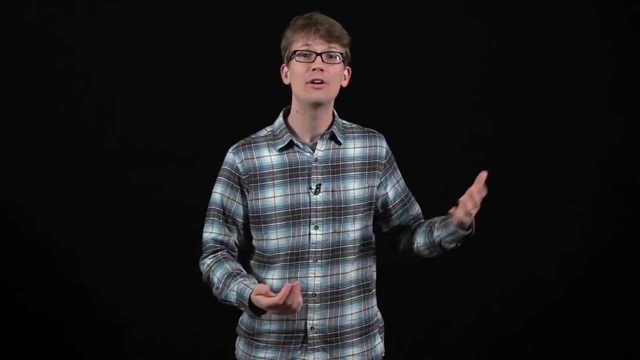 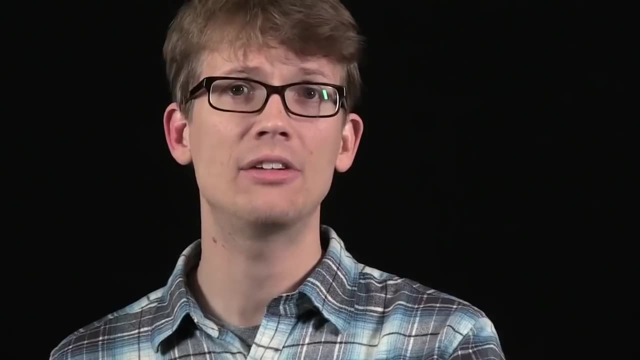 causing erosion and washing minerals and chemicals all the way to the sea, where it affects marine ecosystems. and when I say effect, I don't mean in a good way. This, my friends, is what's called a cascade effect, in this case caused by deforestation. 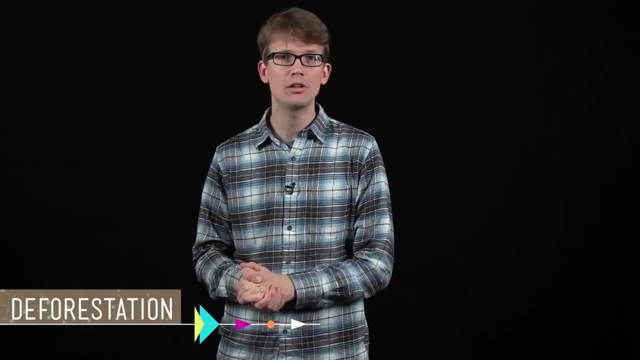 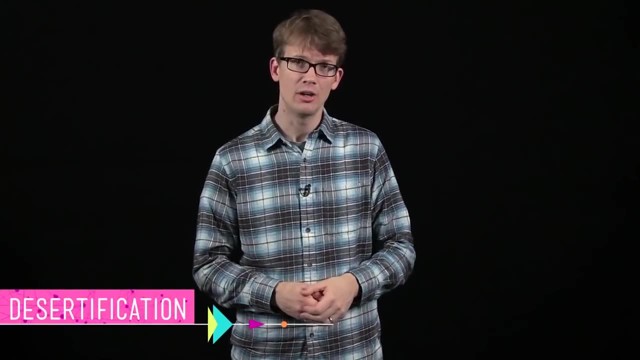 one of the most obvious observable human impacts. In addition to causing more flooding and changes in water quality, deforestation on a large scale can lead to another impact: desertification or the spread of dry, unproductive landscapes. But cutting down trees doesn't automatically turn a forest into a desert. Desertification is driven along by additional factors like overgrazing by cattle and over-irrigation. So how can over-watering something make it turn into a desert Well? when we use groundwater to irrigate crops, the natural salts in the groundwater build up in the soil. 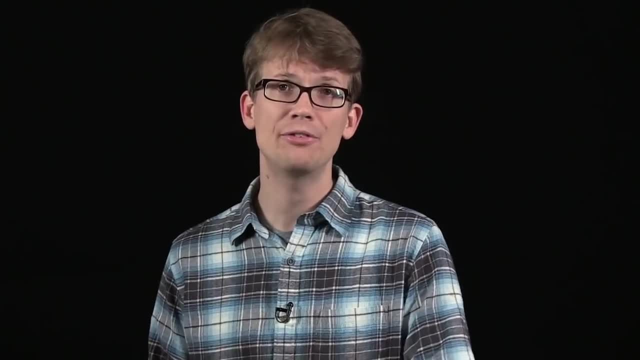 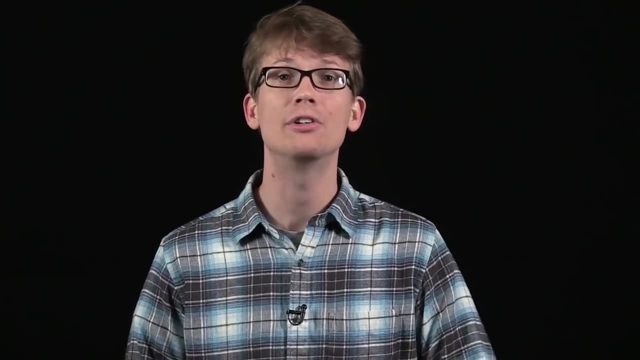 eventually making it so salty that nothing wants to live there. Over time, fertile land near desert ecosystems become overtaxed and the desert spreads. And this is exactly what has happened in China over the past century, where overgrazing and the city's unquenchable thirst for water 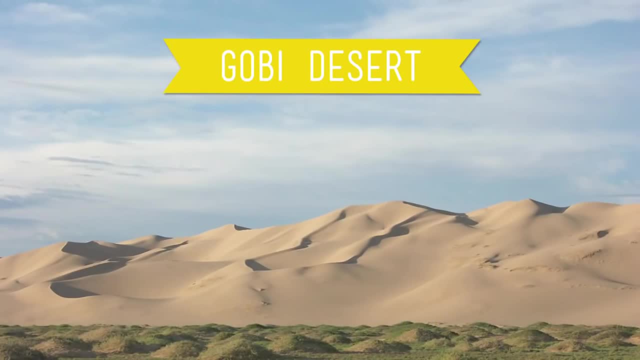 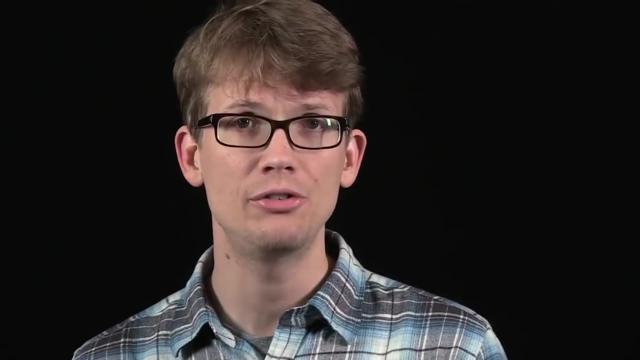 have caused the Gobi Desert to grow by 3,600 square kilometers every year. Now, these two impacts by themselves clearly limit the biodiversity of otherwise lush ecosystems, but because they also result in fewer trees that provide the all-important services of releasing oxygen. 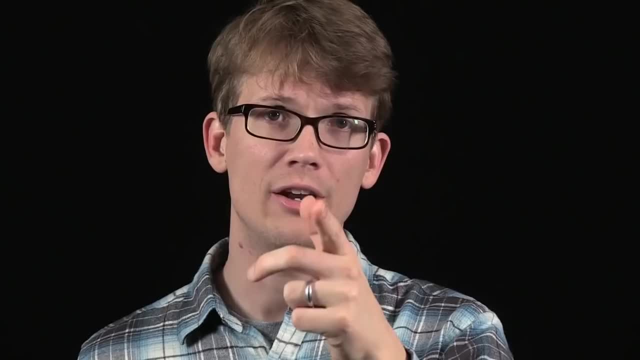 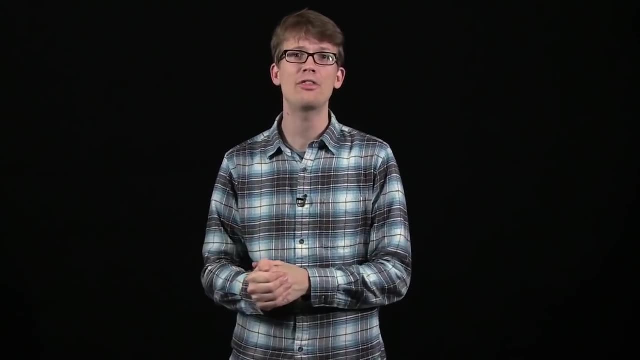 and absorbing CO2, you know what domino's gonna fall next? The climate. Carbon dioxide, the principal greenhouse gas. it insulates the Earth. so it stands to reason that the more CO2 there is in the atmosphere, the warmer the Earth will be. 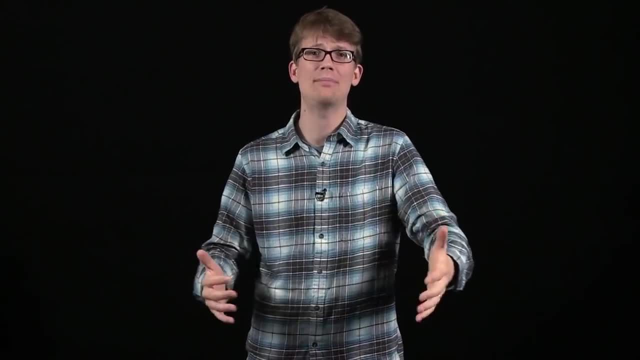 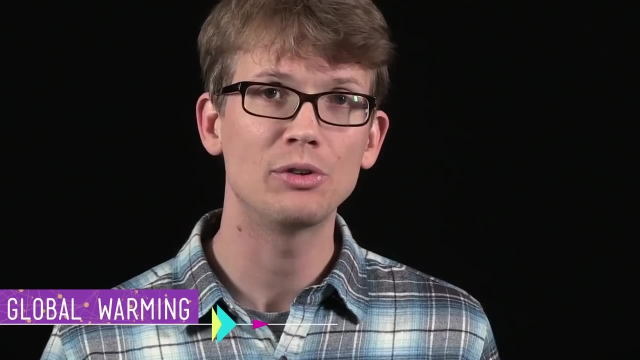 And the thing is, we're reducing the size of forests at the same time as we're unleashing all kinds of greenhouse gases by burning fossil fuels. This double whammy is much of what's driving global warming. As a result, we're seeing decreases in the levels of polar sea ice. 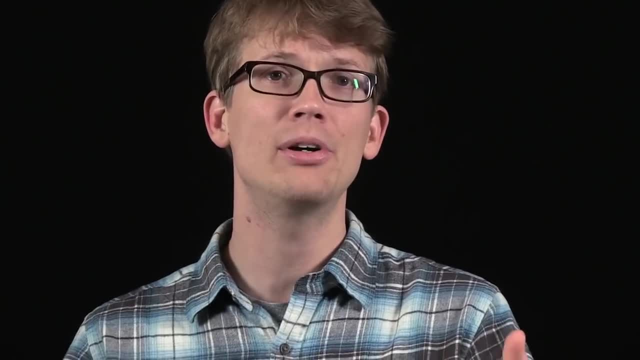 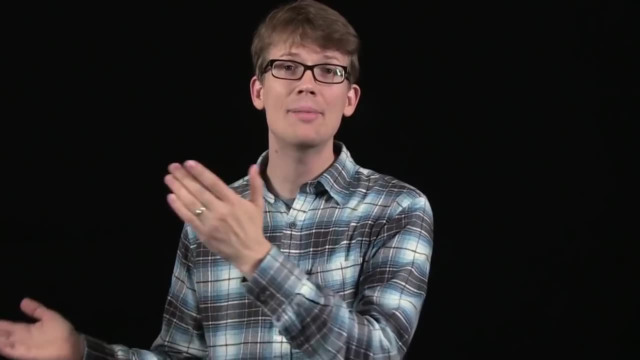 which means less habitat for polar bears, seals and seabirds. more temperate animals are moving closer to the poles, and hotter, drier conditions are causing more grass fires and forest fires. And while the climate has changed many times in the past, 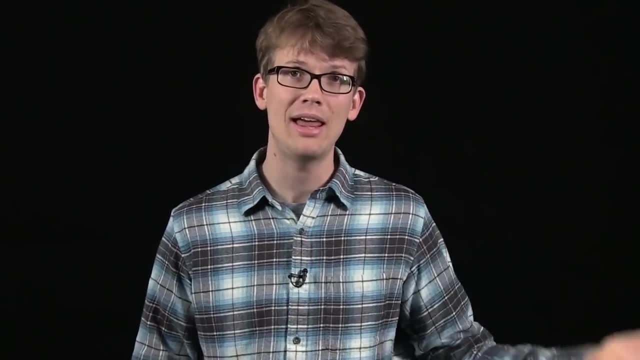 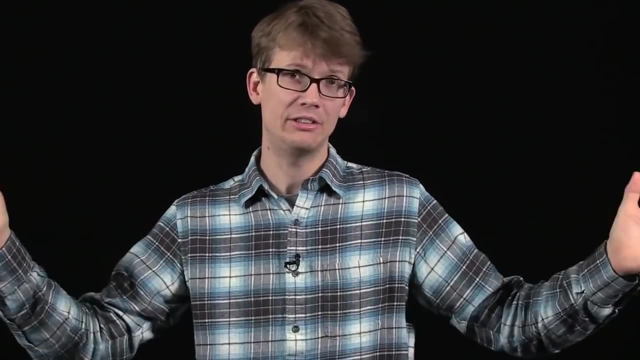 those changes usually took place over centuries or even millennia, giving organisms time to adapt or move. These changes are taking place within our lifetimes and it's kind of a huge deal and it's complicated. It'd take me at least like 10 minutes and 52 seconds to explain it all in detail. 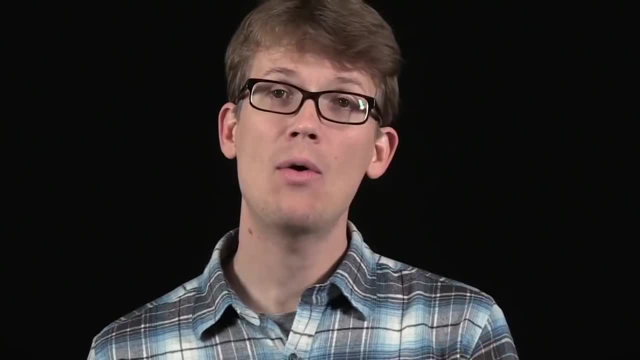 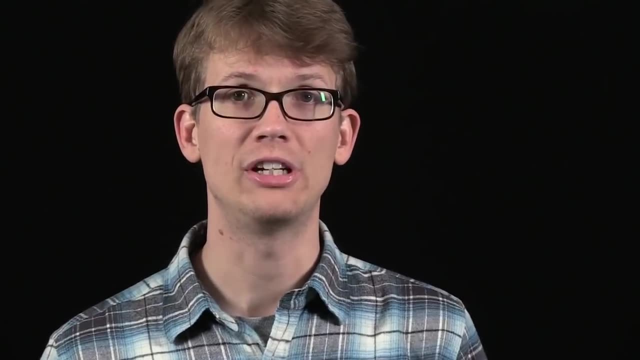 which is why I did that in another video. By now, hopefully, you can see how one huge change in human impact can lead to another and how, even indirectly, they can end up reducing biodiversity. But it's hard to overlook the more immediate impacts we can have on ecosystems. 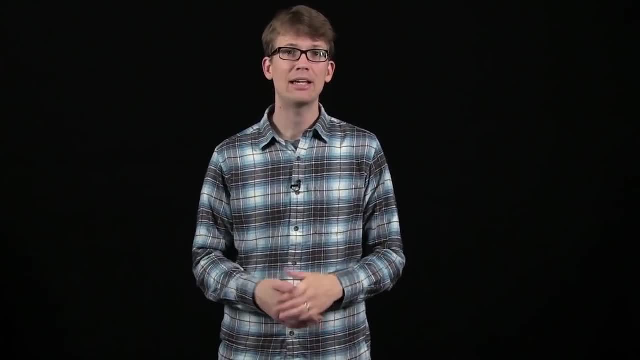 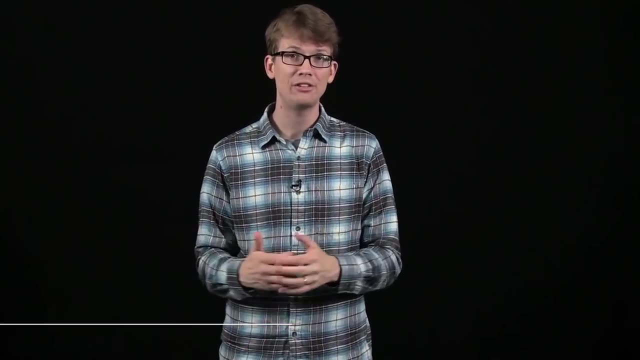 One of the more in-your-face ways we affect biodiversity is by introducing non-native species, either intentionally or unintentionally. Again, there are so many examples of this that you can learn more about it in another video I did, But suffice it to say whether it's kudzu in North America. or cane toads in Australia. invasive species have a knack for out-competing or outright eating native species, to the point that it rocks the world of an entire ecosystem. And finally, probably the most direct impact we have on biodiversity is simply over-harvesting certain organisms. We're overfishing the oceans to meet growing demand for popular fish species like tuna, while on land we're exterminating important predators like wolves to protect livestock- those cows again- And the less diverse those ecosystems are, the more vulnerable they become to disturbances. 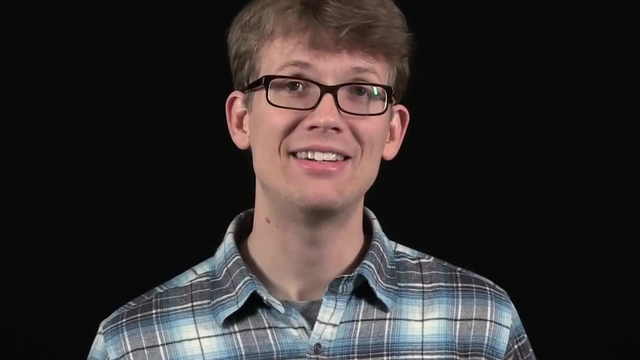 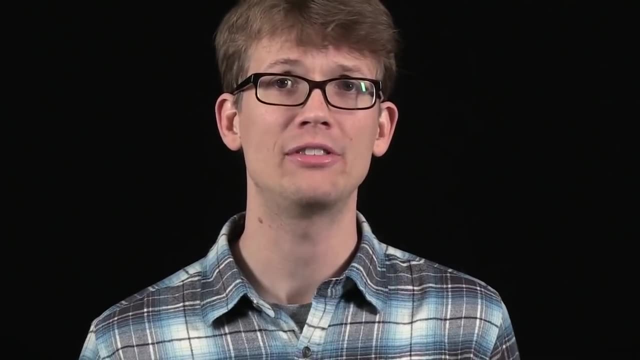 including those other four impacts I just mentioned, And the fact is there's a bunch more where those came from, because there's a whole separate set of effects that humanity has in the biosphere that stems simply from us putting the wrong amounts of certain stuff.